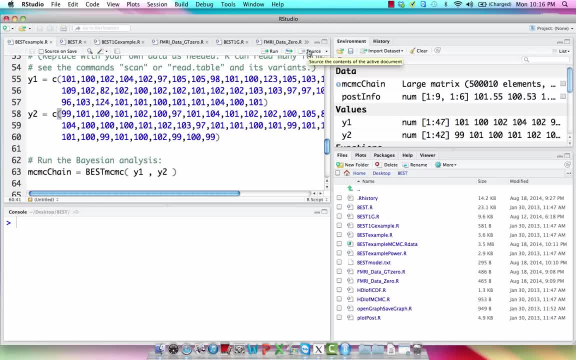 this is what makes RStudio very efficient, very quick and easy to use. So if I click on that, it's basically like I just copied and pasted all the text in this file right here into my console down here. So right now it's already run the burn-in, just like in that web app where we had the burn-in samples. So if you didn't run the burn-in, you could run the burn-in. but if you didn't run the burn-in, you could run the burn-in. but if you didn't run the burn-in, you could. 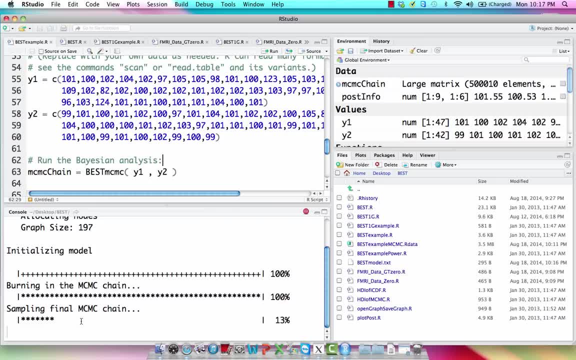 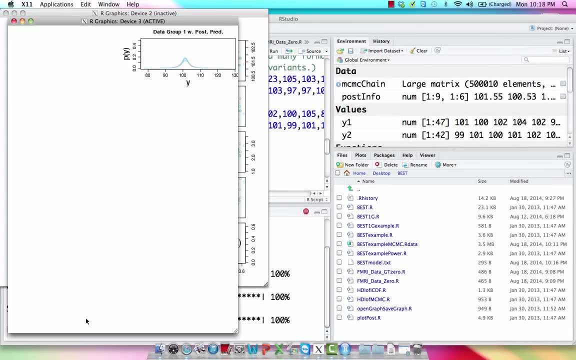 discard and now actually sampling the MCMC chain. This takes a little while and instead of having a really long awkward silence, I'm just going to make the screen go blank until the MCMC chain is finished sampling. All right, now that the sampling is finished and we've built up our 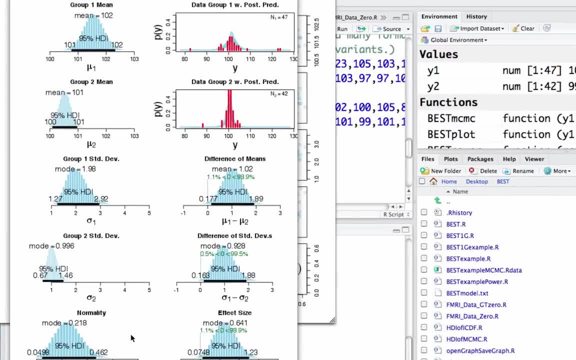 posterior distributions. this function also automatically plots all of these different parameter estimates for you. So notice, just like in the web application, we have different parameter estimates and also this 95% HDI representing the density, the highest density interval of our parameter estimates. Okay, so we have individual group mean estimates, standard. 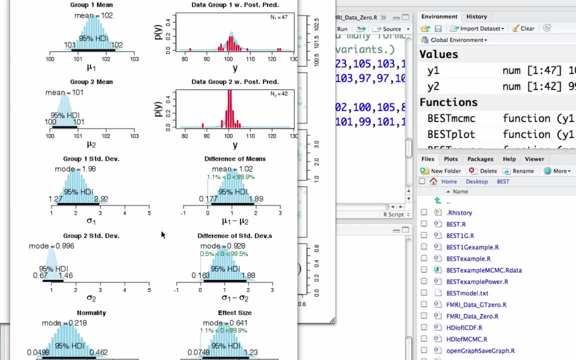 deviation estimates, normality estimates, effect size and probably what you're most interested in, since we are comparing groups, is an estimate of the difference of means. Notice that Bayesian inference is very robust against things like outliers. We can see some of the raw data plus. 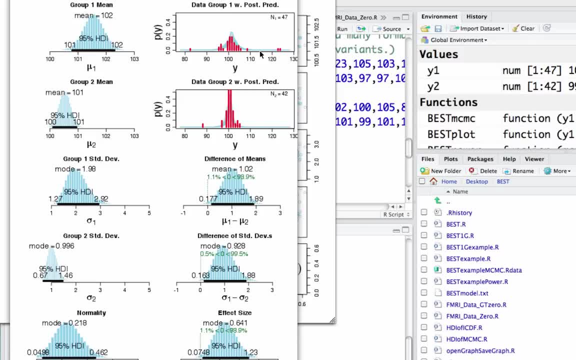 plotted in these red bar histograms right here. So even though we had quite a few outliers, really that didn't affect our parameter estimate that much, And even though we had unequal group sizes, it also did not pose much of a problem. Bayesian inference was very robust against what would 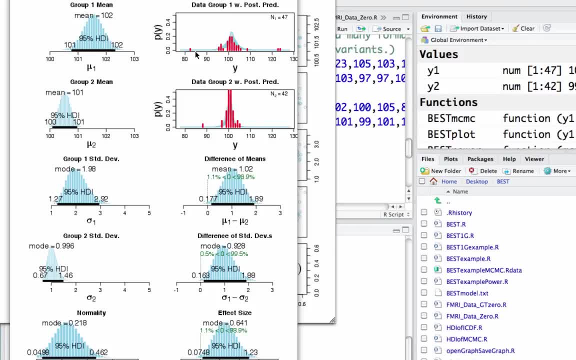 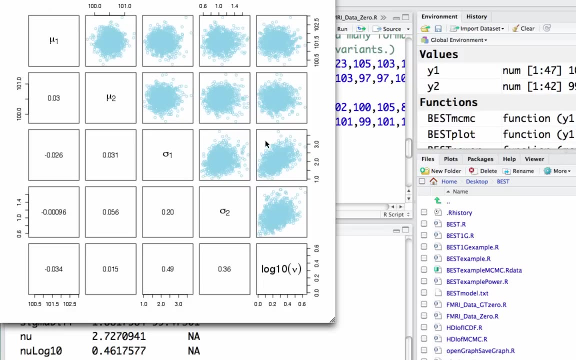 typically be problems for running t-tests. Okay, so that is basically the equivalent of an independent samples t-test. Really, we're just doing Bayesian inference for a group difference, but we're also doing it for a group of means. Okay, you also get these plots which show: 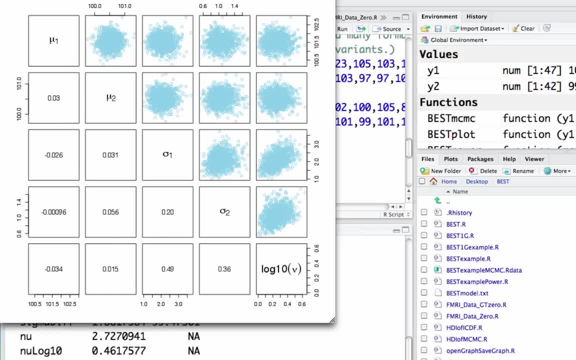 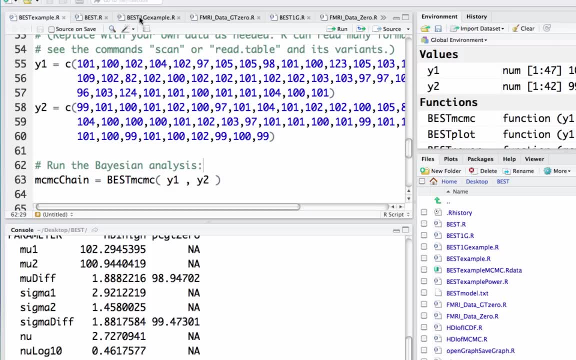 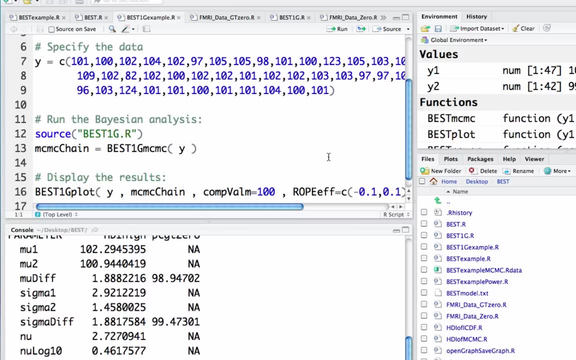 correlations between different parameters, which also provides you information about that. Okay so that's a topic for another time, but that information is there for you to peruse if you wish. Lastly, I want to show this best 1G example. Okay so this is basically one group And, critically, 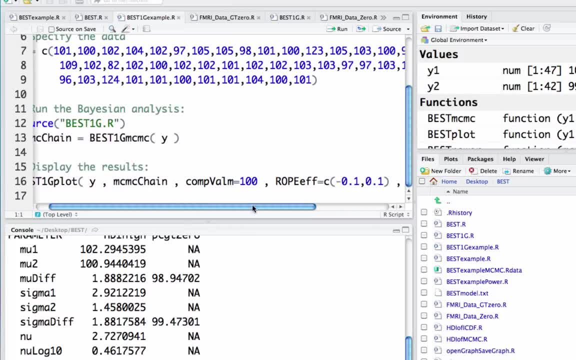 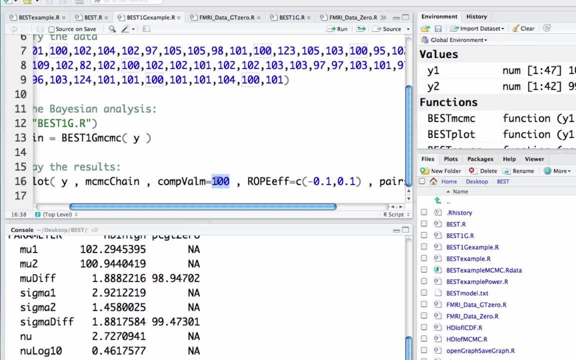 here is something that we're going to want to change: This comp val m. this is the mean that we're comparing to. So if we're, basically, if we just have one group, what are we? what are we trying to compare it against In a lot of cases, you know. 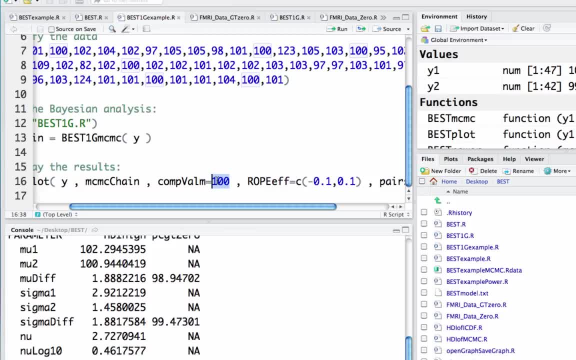 if you just have the differences from a paired groups test, you might be comparing this to zero, which would basically compare it against a null value, which says that there is no difference between them. So I'm going to go ahead, run the source here. let's bring in the MCMC chain. 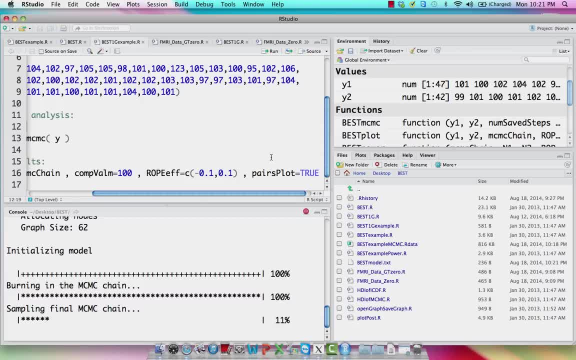 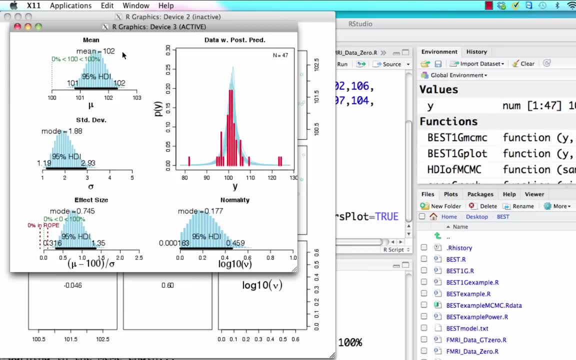 and again, I'll just take a few seconds timeout Until this thing finishes. Okay, the sampling is now finishing up And, again, just as before, we now get some plots showing these different distributions. Okay, so notice that we now have. 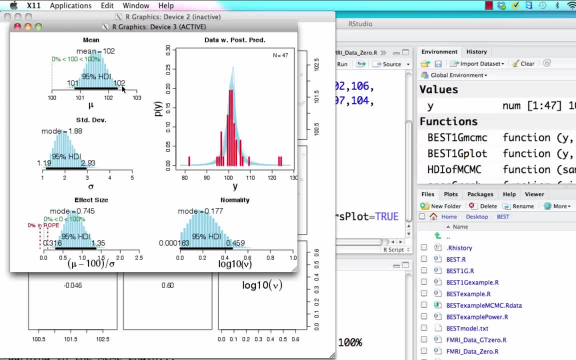 an HDI spanning values from 101 to 102.. And also notice that this entire HDI falls well outside of a value of 100.. So if we're comparing this to a value of 100, and we also had a rope just around- 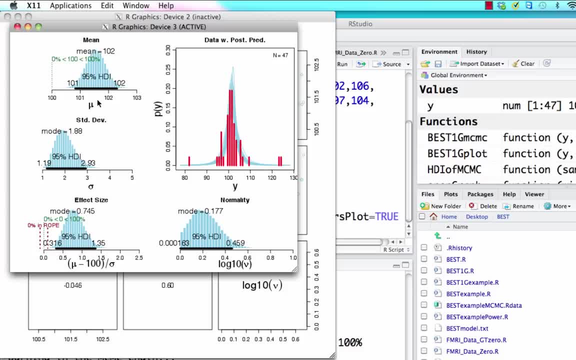 it and we're comparing this to a value of 100, and we also had a rope just around it and we're a very narrow band of that interval. right there, we can go ahead and say with confidence that our parameter estimate appears to be within this region and not include this value down here. 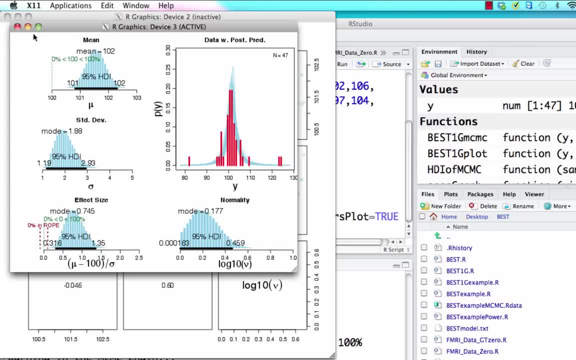 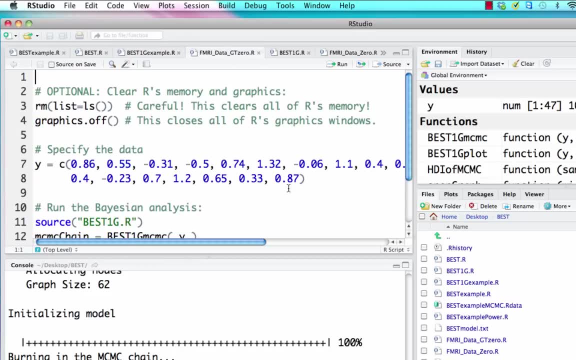 And we also have a rope on things like different parameters such as effect size. The last thing that I want to show you guys is an example that I would apply to some, say, fMRI data. I do this all the time, So usually when I extract data from a region of interest. 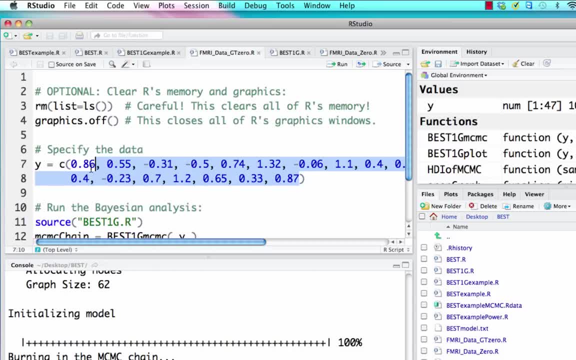 I now have things like signal change or parameter estimates, contrast estimates. what have you? And usually with fMRI data you get values roughly within say the negative point 1 – or say negative 1 to positive 1 range. 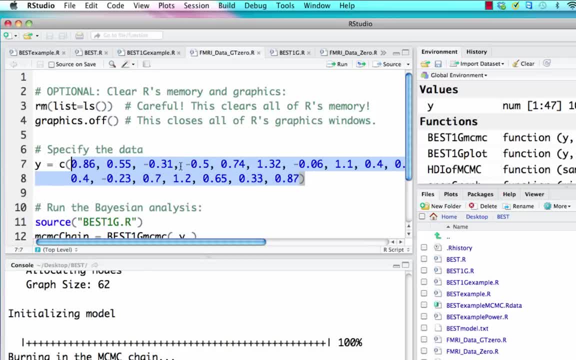 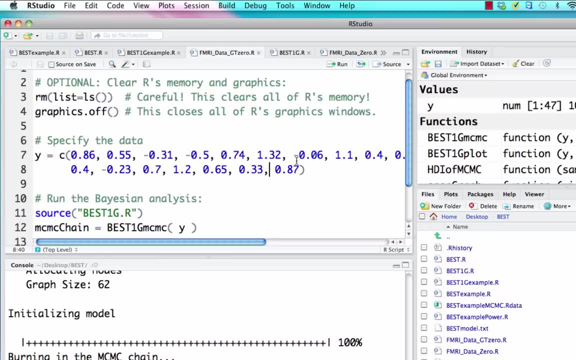 And let's say I collect data from – I think this is close to about 20 subjects and I want to see whether this is actually different from 0. Okay, whether my parameter estimate is credibly different from 0. And not only that, but I might be. 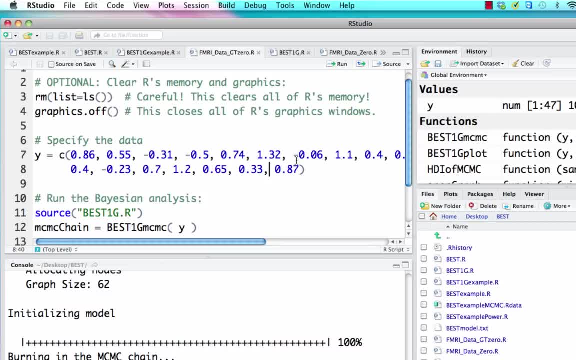 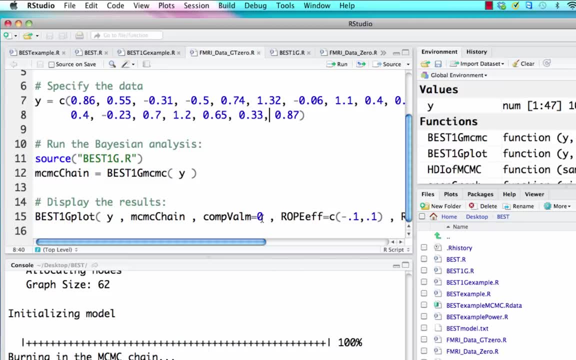 interested in actually trying to see whether 0 is among the credible values of my parameters right Now. notice: what I would change here is: first of all, I would change all the data within this vector. I would also change conflm to 0, since that's usually what I'm trying to compare against And a good rope is about. 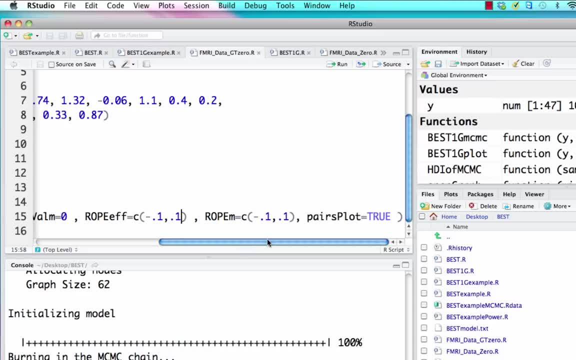 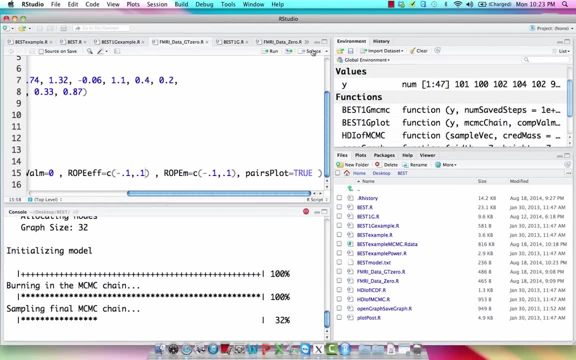 0.1, or negative 0.1 to 0.1.. Okay, I'm going to go ahead and run this. This is actually quite quick, So I'm just going to leave this up here. Last thing: notice rope EFF. that's for the effect size and rope M is for the. 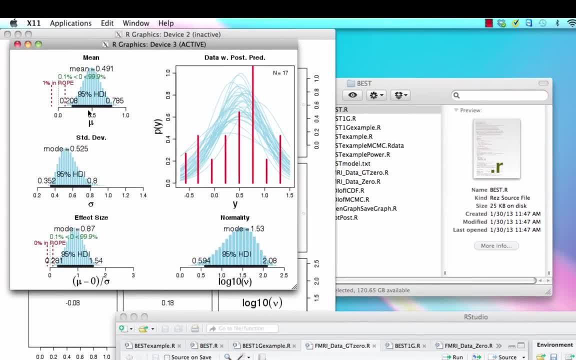 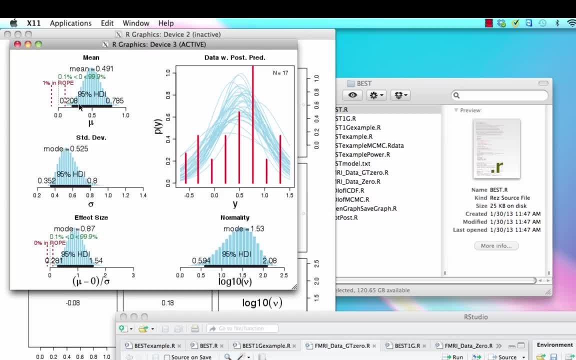 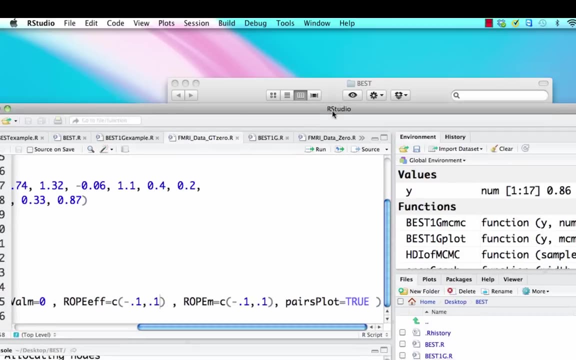 HDI falls outside of the rope, suggesting that my credible parameter value is actually well outside of this region of practical equivalence, which I would put for a null value of 0.. And lastly, also, we get these plots that show correlations between parameter estimates. One more example, again with some just 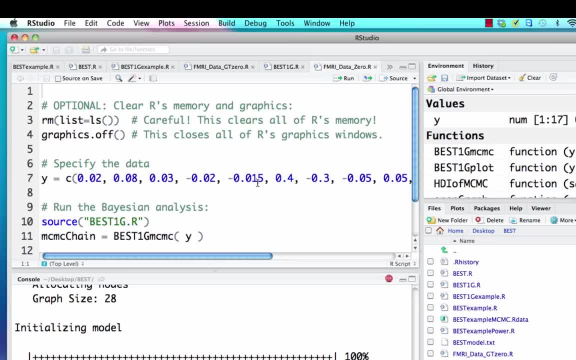 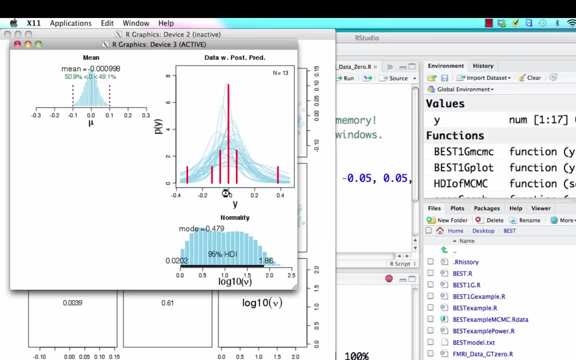 sample data right here is what if we're actually trying to show that the data supports a null hypothesis? Again, this is basically impossible to do with traditional NHST methods. But in this case, let's say I have a bunch of values which appear to be around 0 and I established a region of practical 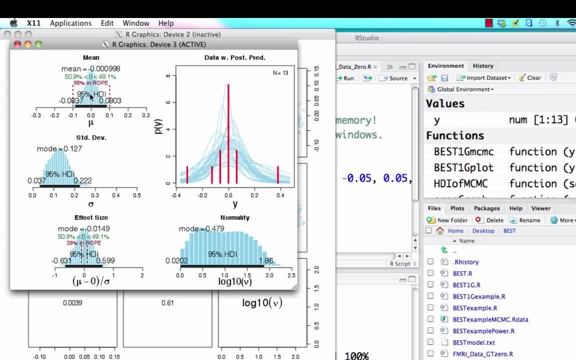 equivalence running from negative 0.1 to 0.1.. And lo and behold, my 95% HDI actually falls well within that region of practical equivalence And in this case I could go ahead and accept what's essentially a null value of 0.. And 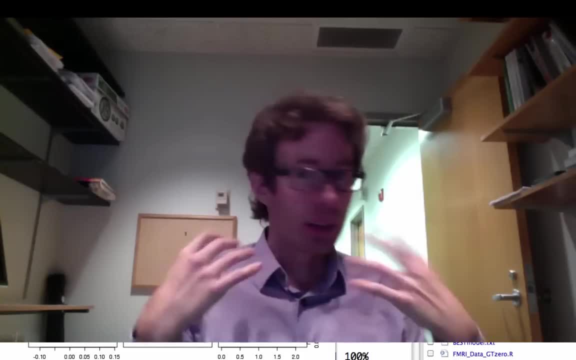 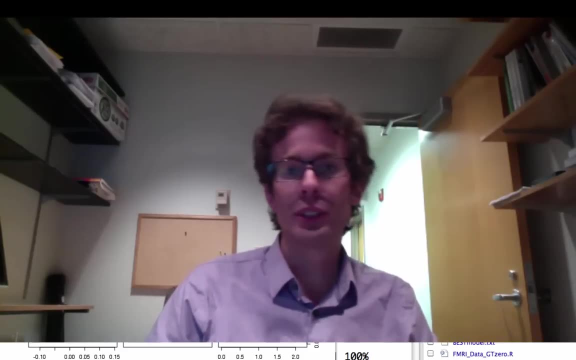 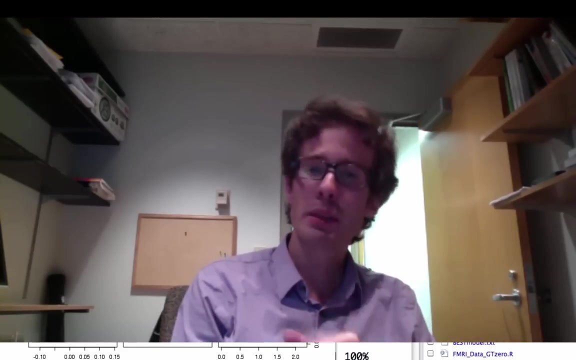 so that's how you do it Again, very simple. you just replace what's in those vectors with the data you collect from your own experiment, And a lot of the Bayesian inference is run for you. The things that you would probably just change are things like your comparing value. So like the mean comparing.